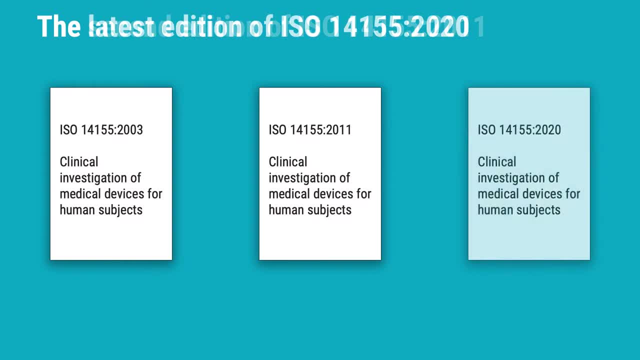 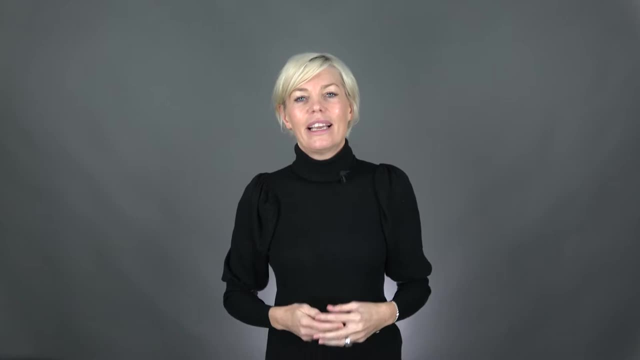 revision of the standard was released in 2011, and the third and current version of the standard was released in July 2020.. This course is based on the 2020 version of the standard. The ISO 14155 standard is an excellent guidance document and I encourage you to carefully read it and understand. 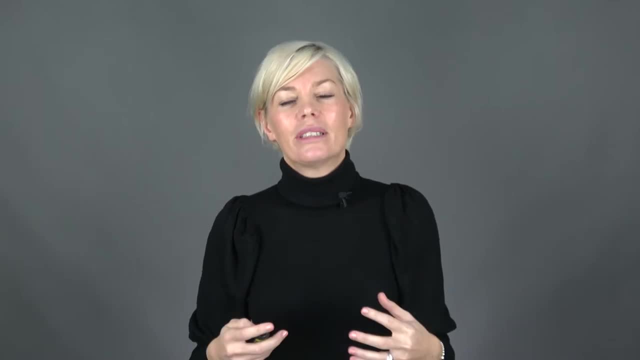 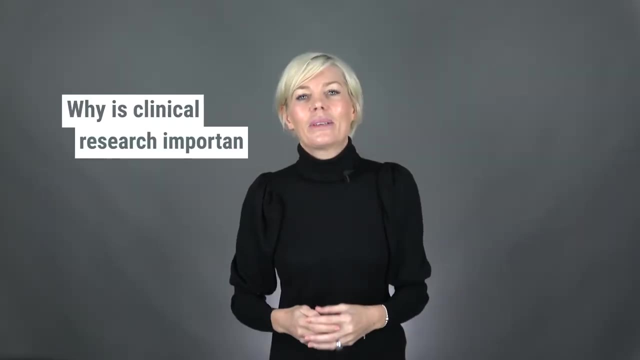 it. It will almost guarantee that you will set up and conduct clinical studies with high regulatory compliance and high scientific credibility. So let's look at what clinical research is and why it's important. Clinical research is necessary to develop new treatments for different diseases and 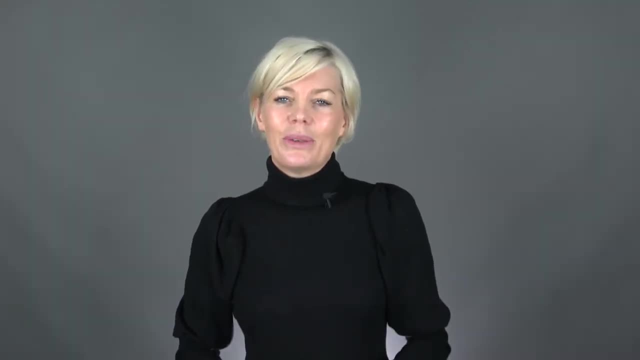 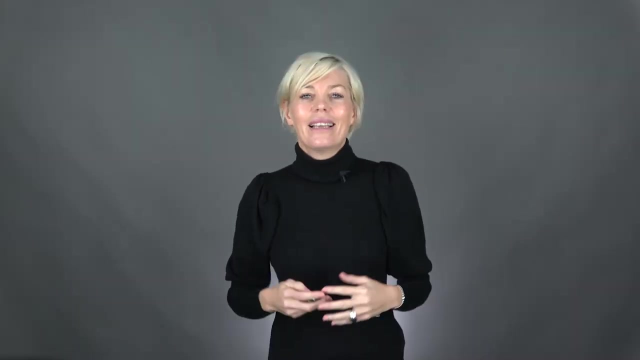 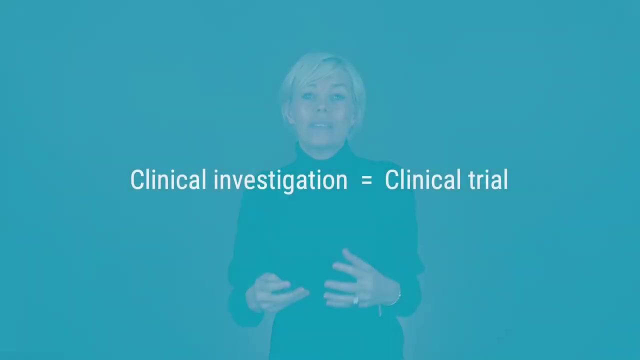 conditions that occur in humans. To develop these new treatments, we have to perform clinical studies to get proof that the new treatment works and that it's safe in humans. Clinical trials and studies using medical devices are called clinical investigations In the ISO 14155. 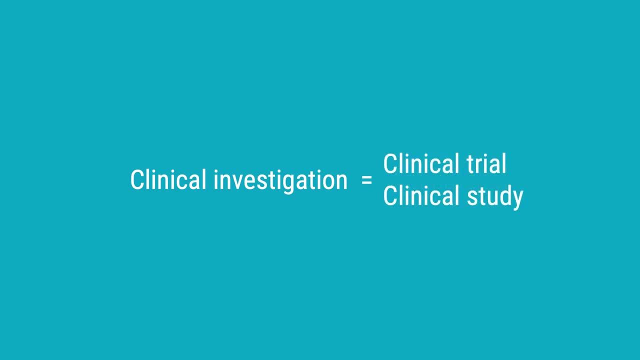 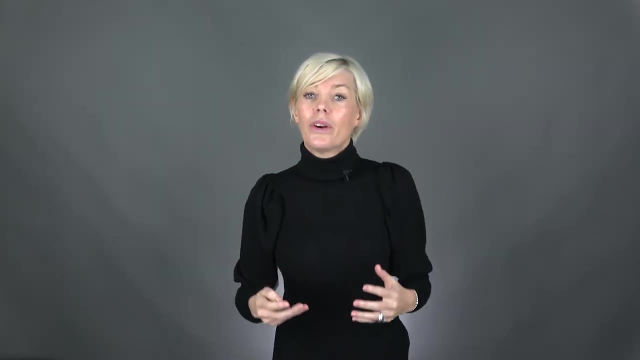 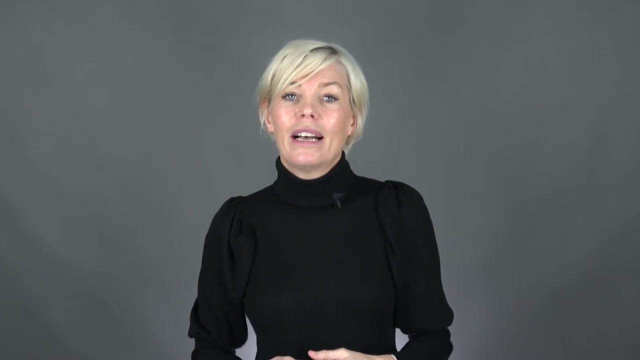 standard, the term clinical trial or clinical study are synonymous with clinical investigation. So clinical investigations are carried out to assess what works and does not work as treatment in humans And, more elegantly, this is described in the ISO 14155 as clinical investigations is. 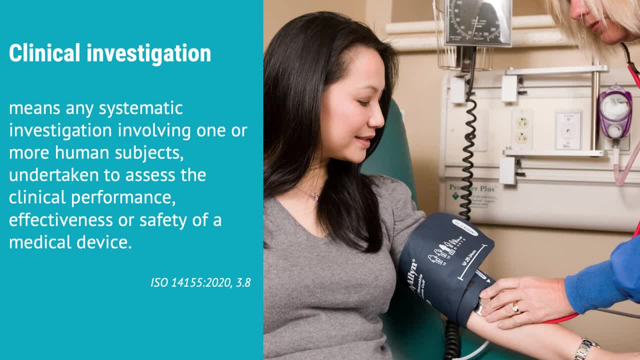 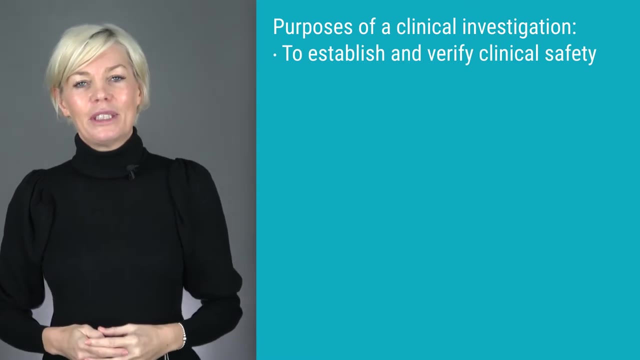 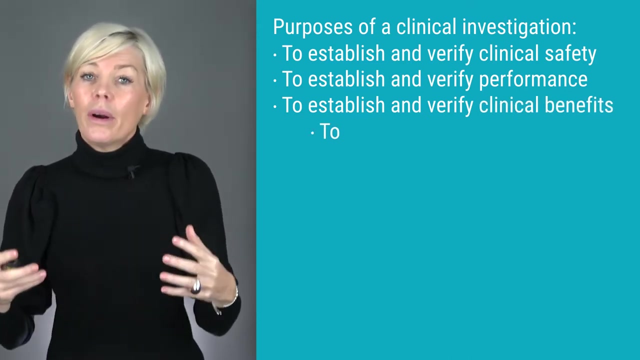 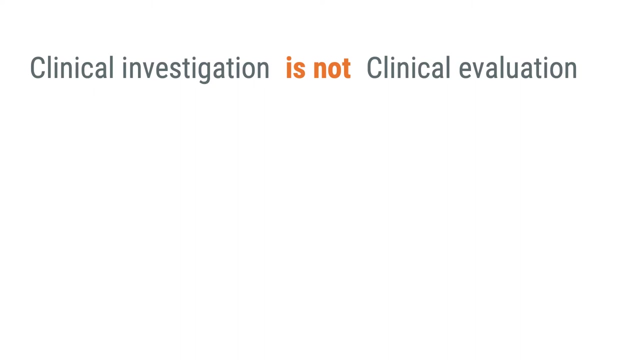 defined as any systematic treatment that is performed in humans. So the purpose of the clinical investigation is to establish and verify clinical safety, or establish and verify performance, or establish and verify clinical benefits or detect any undesirable side effects. I want to emphasize that clinical investigation should not be 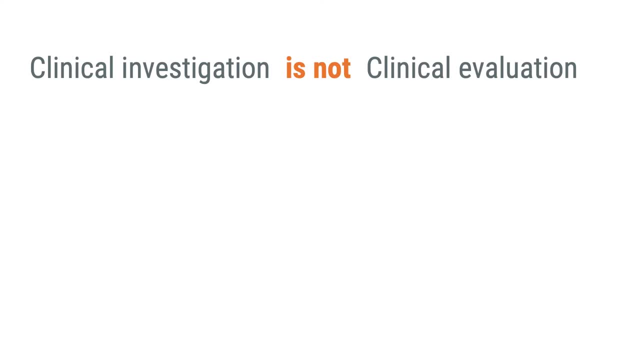 confirmed by a clinical study. If a clinical study is not confirmed by a clinical study, it is a technical evaluation. If a clinical study is not confirmed by a clinical study, it is a clinical evaluation. It is easy to misuse or use the terms interchangeably, but it's important to 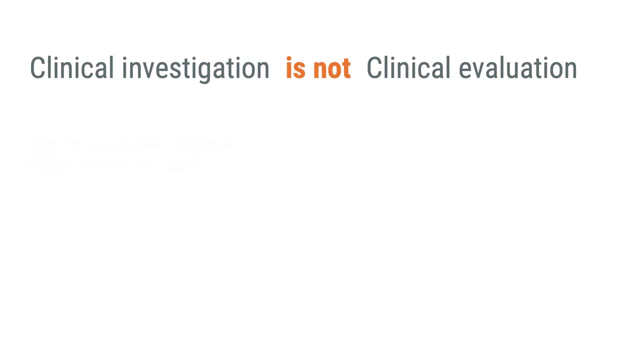 know the difference, so we know if we speak about one thing or the other. So, in other words, a clinical investigation is when you're using a medical device on real patients to demonstrate the safety and performance of that medical device, Whereas a clinical evaluation is a theoretical and 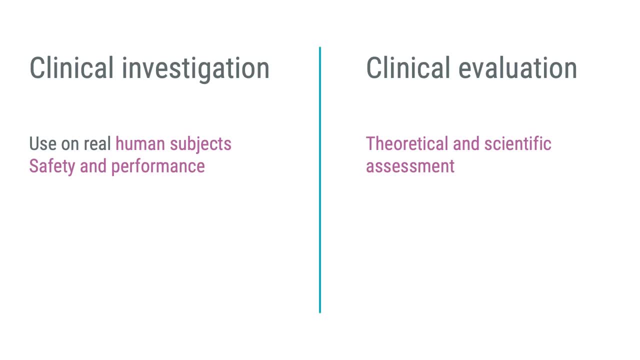 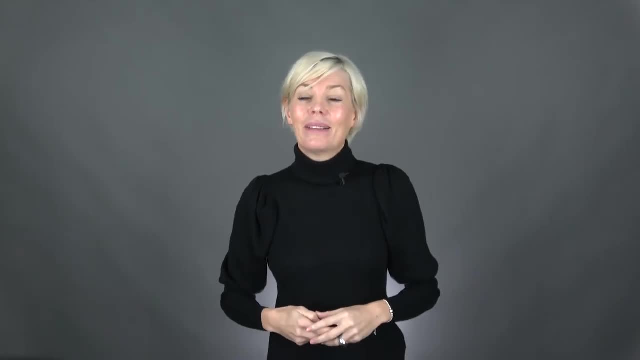 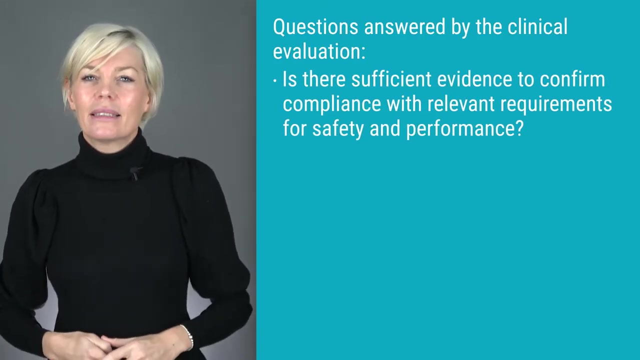 scientific assessment of existing data from many different sources, So it's important to know the different clinical investigations and other sources of clinical data. Furthermore, the clinical evaluation is about answering two important questions, such as: is there sufficient clinical evidence to confirm compliance with relevant requirements for safety and performance when using? 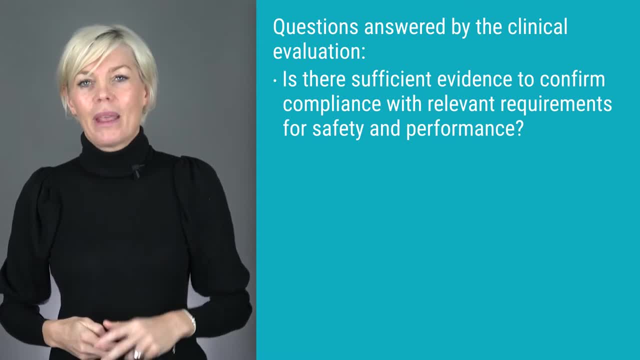 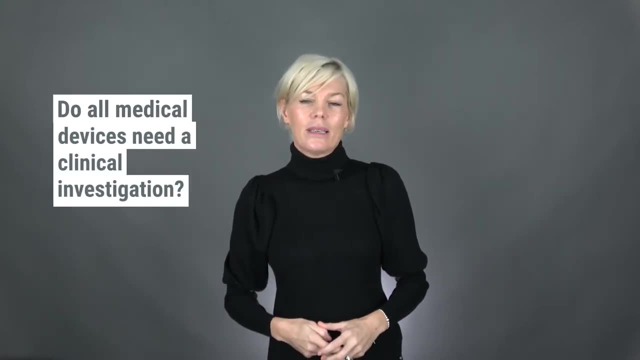 the device according to the instructions for use. There are a few And is a clinical investigation needed. Now let's look a bit more in detail at clinical investigations. So do all medical devices need a clinical investigation? Well, here it's important to make a 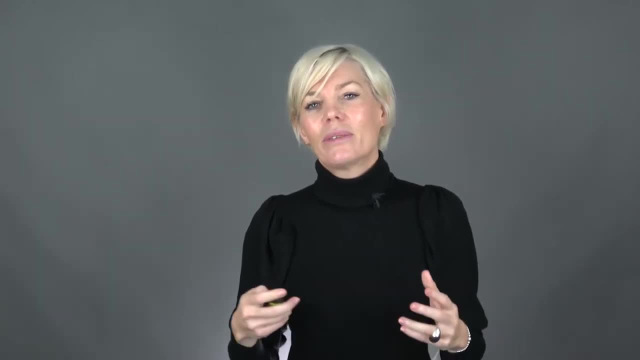 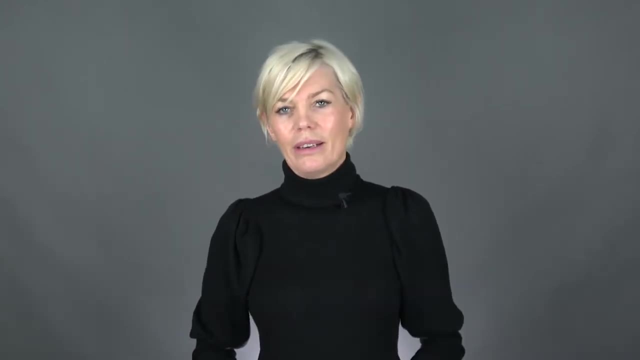 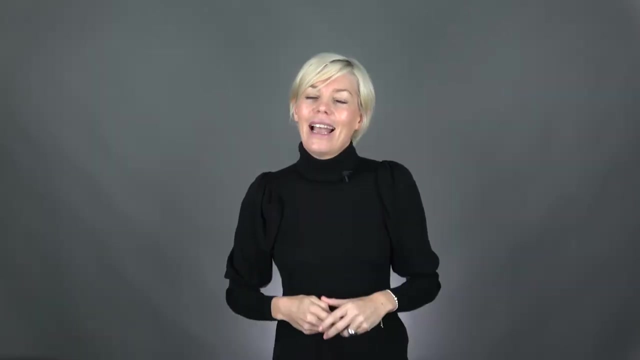 distinction between clinical research of drugs and clinical research of the devices. So, when studying new drugs, a clinical trial is always required. However, when studying medical devices, a clinical investigation may be required, And this decision is based on the novelty of the device. 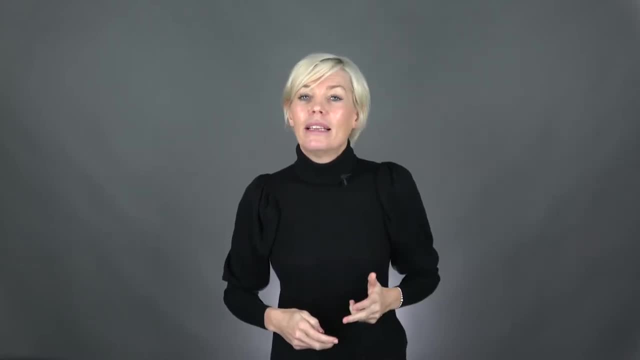 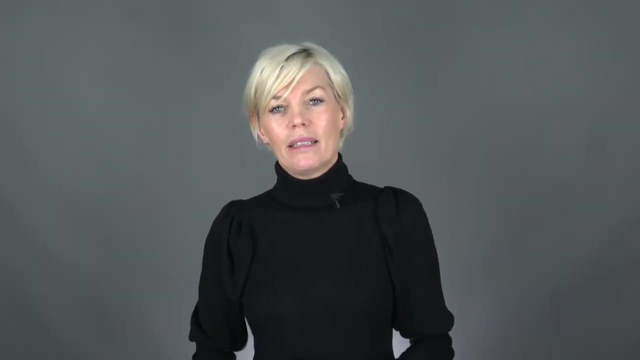 the risk classification of the device, the outcome of the clinical investigation and the necessary medical efficacy. And what is the risk classification, evaluation and the conclusion from the risk analysis of the device? You may think that why wouldn't all new medical devices need a clinical investigation? 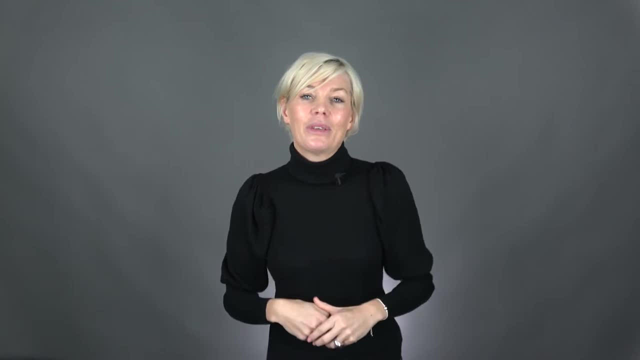 How can you know that they're safe? Well, if you're manufacturing a syringe or a scalpel, it might be possible to say that the device is safe and performs well by using results from relevant preclinical testing of that device, including bench tests, in vitro, tests, ex vivo. 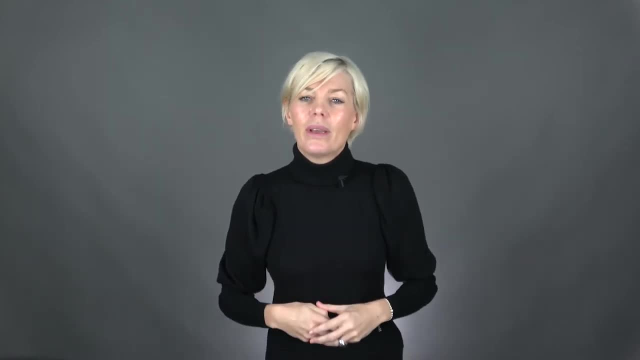 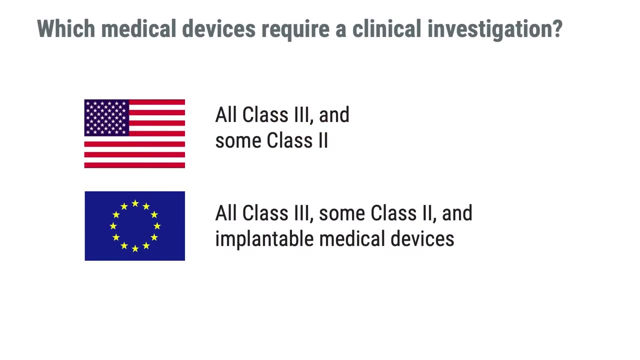 tests, animal tests and so on, together with an evaluation of published literature on that device. Nevertheless, in the United States, all high-risk medical devices, such as class three devices and some class two, require a clinical investigation In the EU, the European Union. 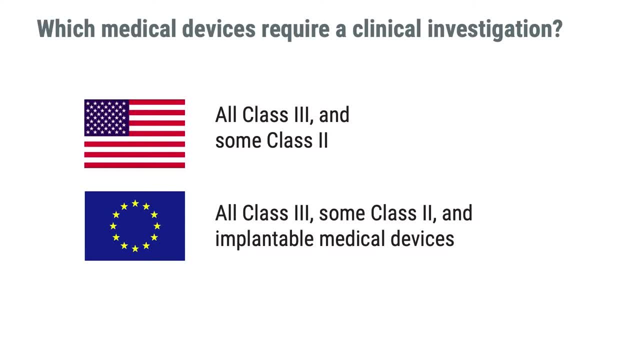 all high-risk devices, such as class three devices and implantable medical devices, require a clinical investigation. Some class two devices require clinical investigation too. There may be some exceptions to this, and in our course on seal marking of medical devices you can learn more about how to classify the risk of a medical device. 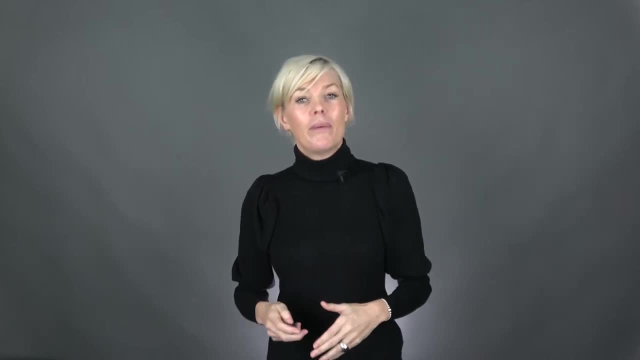 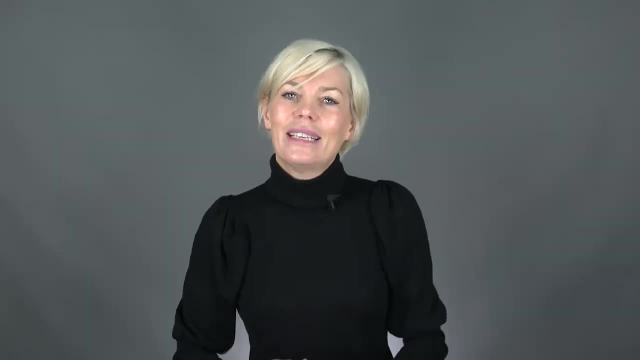 Now that you know more about what clinical research is and what clinical investigations are, let me bring you up to speed on what good clinical practice is. So good clinical practice, also known as GCP, is an international quality standard that describes how to manage clinical trials involving human subjects. Governments can use this standard to transpose it into. 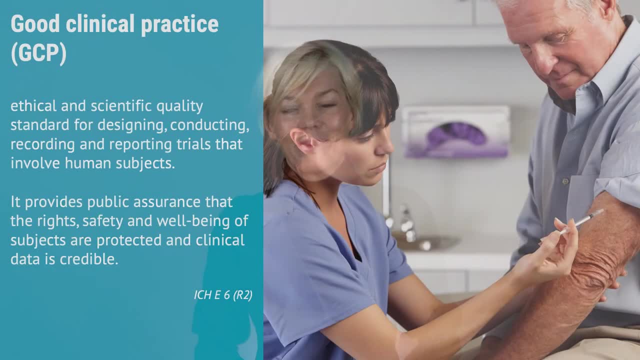 regulations for how to set up and manage clinical studies. The GCP standard is an ethical and scientific quality standard for designing, conducting, recording and reporting clinical trials that involve human subjects. It provides public assurance that the rights, safety and well-being of subjects are protected and that clinical data is credible. The GCP standard. 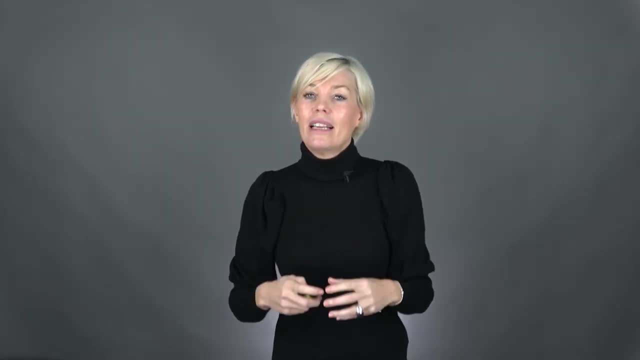 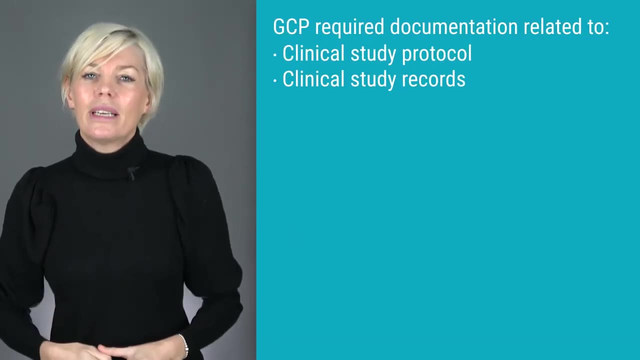 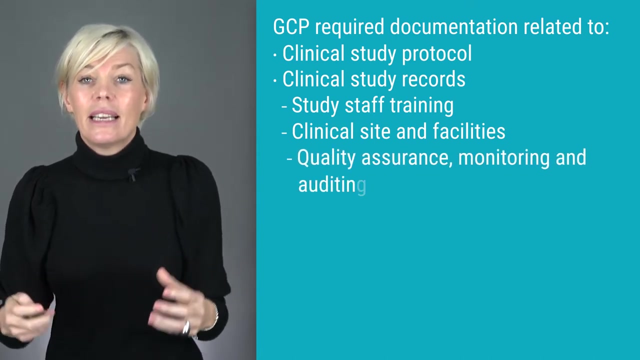 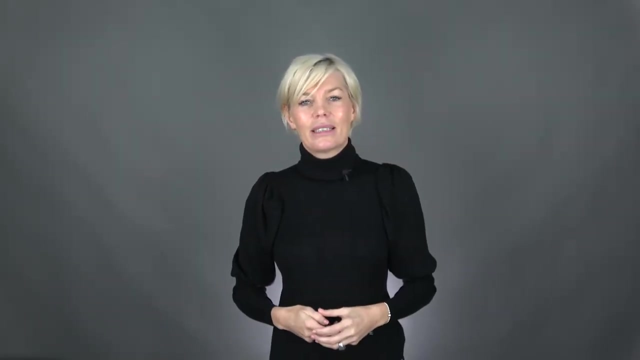 also establishes what is required in terms of how to prepare GCP required documentation, such as a clinical study protocol, how to maintain important records, how to train study staff, how to qualify the clinical sites and its facilities, how to maintain quality assurance and perform monitoring and auditing. You may have seen the acronym ICH in the context of GCP. 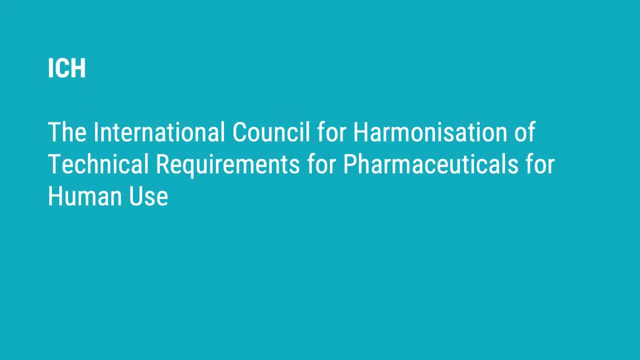 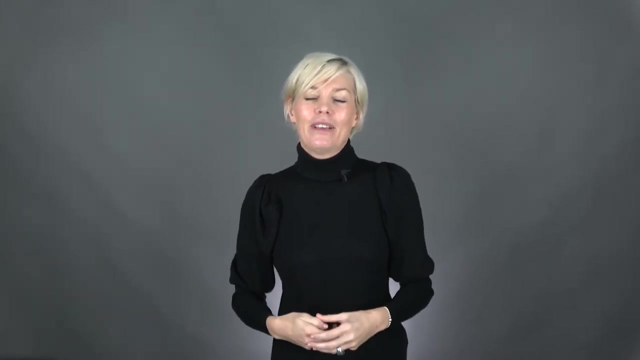 The ICH stands for the International Council for Harmonization of Technical Requirements for Pharmaceuticals for Human Use. Wow, I almost wasted my time there. Anyway, the mission of ICH is to promote public health by achieving a greater harmonization of global drug development. The ICH does this by developing. 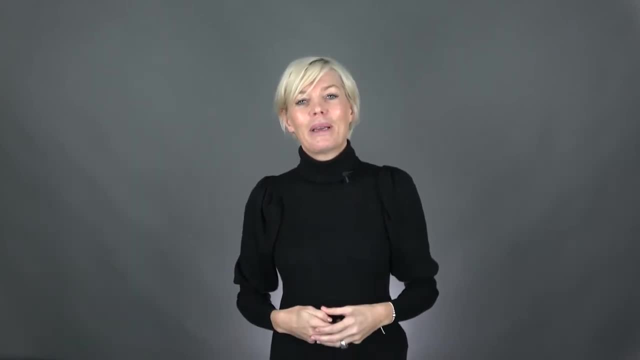 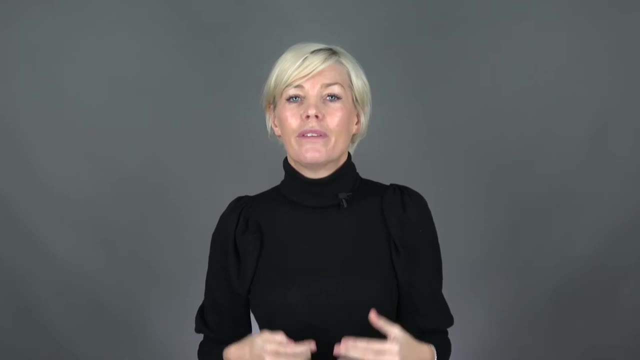 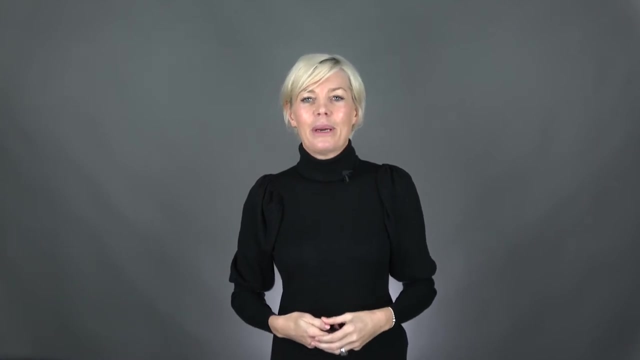 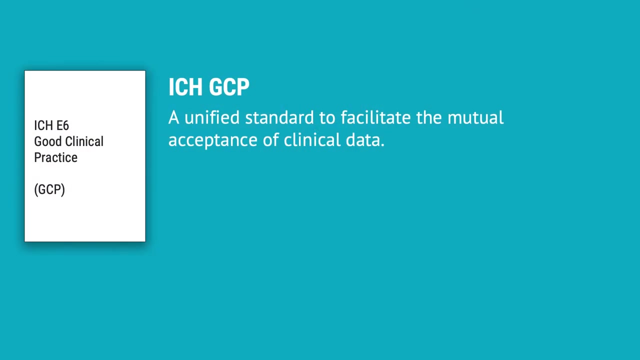 technical guidelines and requirements that can be used by the regulatory authorities and the pharmaceutical industry. Harmonization leads to more rational use of humans and animals and other resources. It aims to eliminate unnecessary delays in the development of new therapies, And that's really great, isn't it? So the GCP follows ICH and enforces 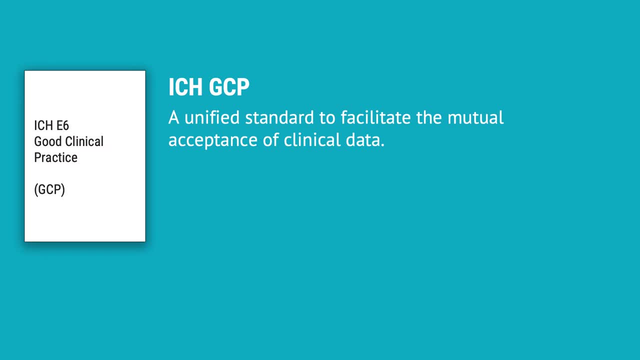 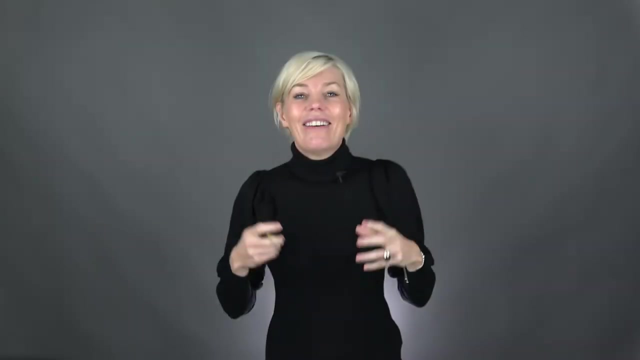 tight guidelines on the ethical aspects of clinical research. The ICH GCP document therefore provides a unified standard for the European Union, Switzerland, Canada, Japan and the United States on how to generate clinical data. Now let's switch to the ICH. 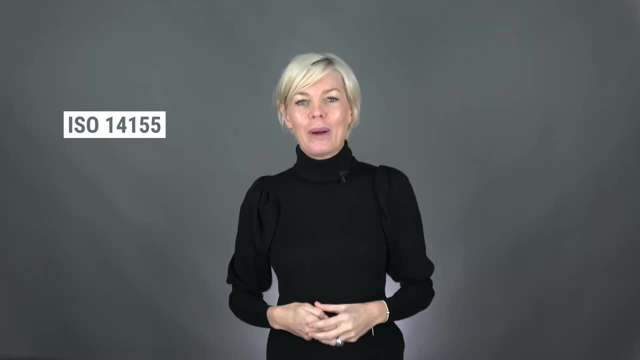 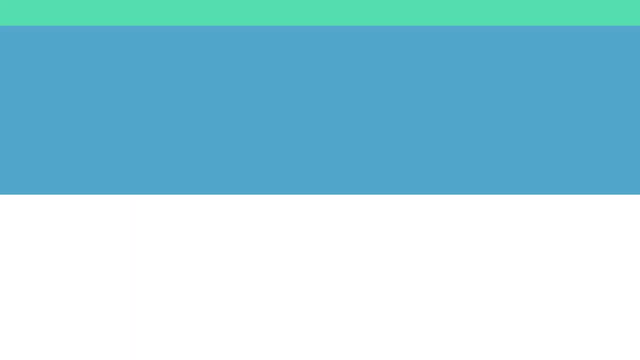 I'm going to switch gears to one of my favorite standards, the ISO 14155.. This standard was specifically developed for clinical investigations of medical devices. It's an excellent tool to help you implement GCP when conducting clinical investigations for medical devices. Similarly to ICH GCP, the ISO 14155 is an international quality standard. 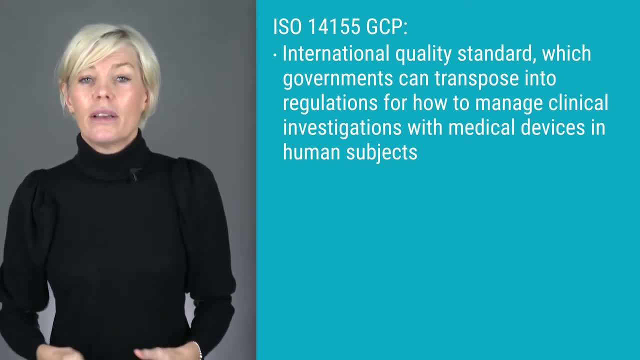 which governments also can use to transpose into regulations for how to manage clinical investigations with medical devices. ICH GCP is a standard that is used to manage clinical investigations for medical devices. ICH GCP is a standard that is used to manage clinical investigations for medical devices. 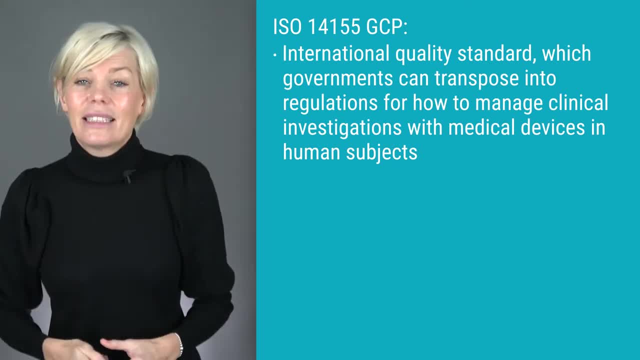 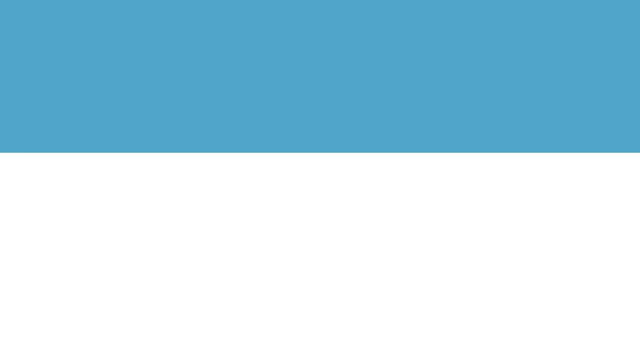 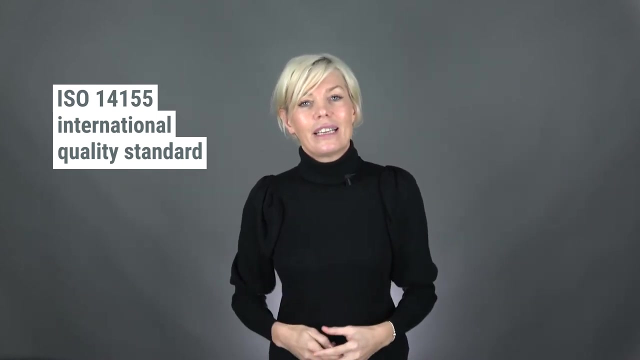 medical devices in human subjects. Just like ICH, GCP, this standard includes protection of human rights for the subjects in the clinical investigation. The ISO 14155 standard provides a detailed instruction on how to set up and perform a scientifically credible clinical study. The standard also helps you understand how to properly document the clinical outcomes. 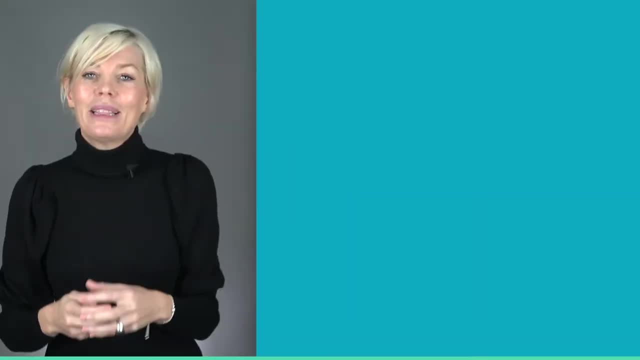 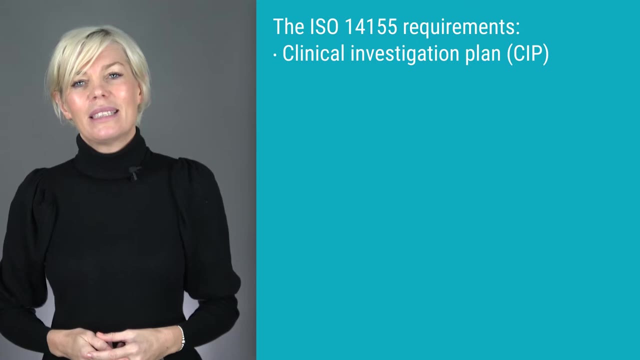 and everything else related to the study. To meet the requirements of the ISO standard, you have to be a clinical investigator. You have to be a clinical investigator have to create a well-structured and complete clinical investigation plan, the CIP. There's even. 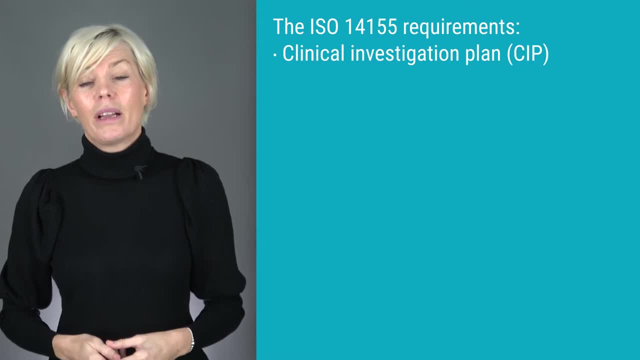 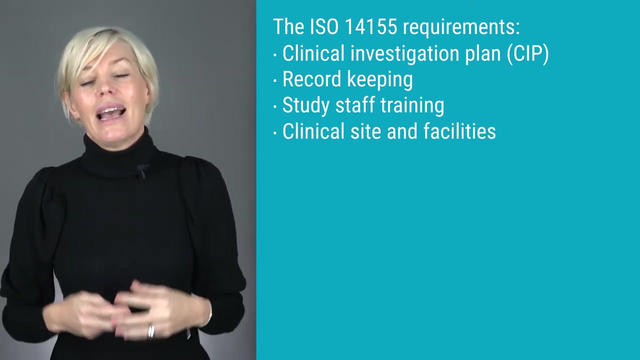 a specific annex to help you with this: Annex A of the ISO 14155.. You also have to keep a good organization of important study documents called records. The standard also describes how important it is to train the study staff and how to qualify the clinical sites and the facilities, And 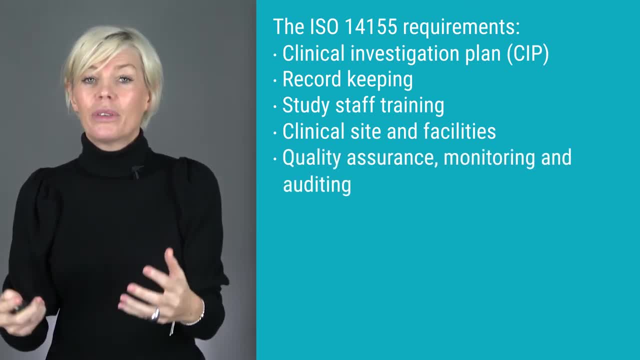 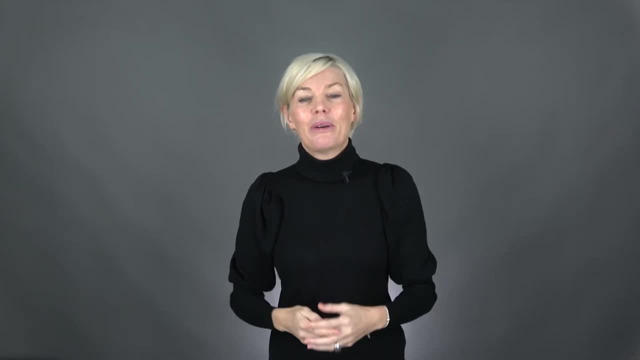 finally, how to maintain quality assurance, performing monitoring visits and how to maintain compliance with the standards. So it's clear that GCP and ISO 14155, the standards are important and that remaining compliant with these standards is essential. But who is responsible to ensure? 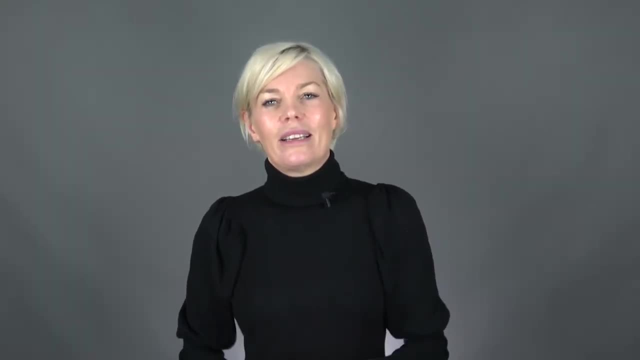 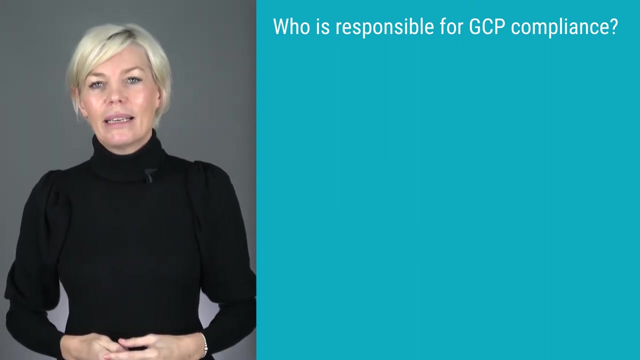 compliance. Let's look at this now. Who are the stakeholders that will ensure good clinical practice and make sure that it's implemented and followed? We will look at the main parties now involved in clinical research. The stakeholders that share responsibility are the stakeholders that are responsible for ensuring GCP compliance. They are the sponsor, the principal investigator. 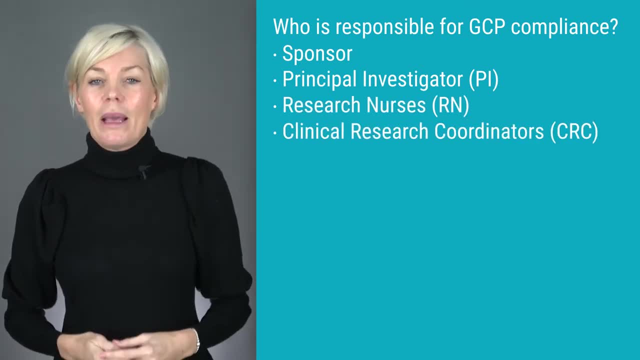 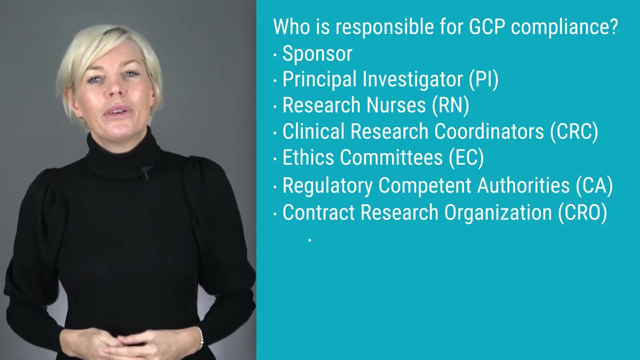 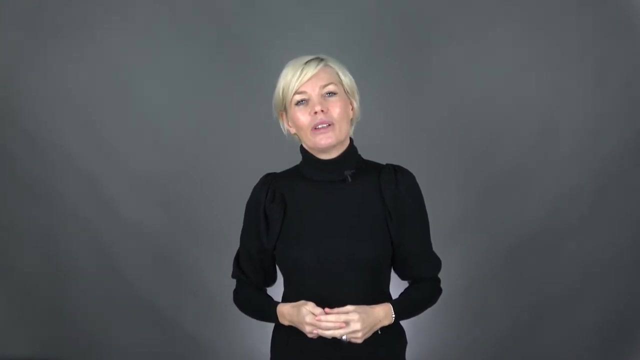 the research nurses and clinical research coordinators. the ethics committees and the regulatory competent authorities. the contract research organizations, CROs and monitors, the medical monitor. All these stakeholders are bound by three basic concepts and duties: Their ethical, scientific and administrative responsibilities. 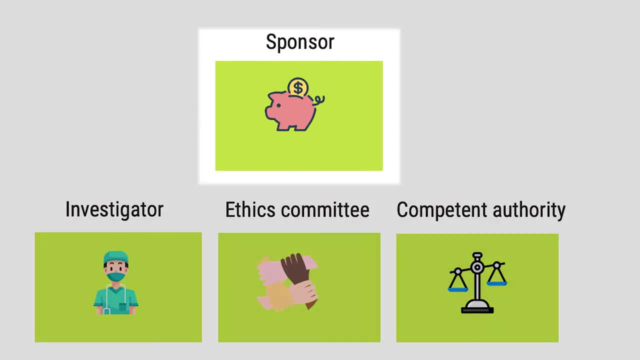 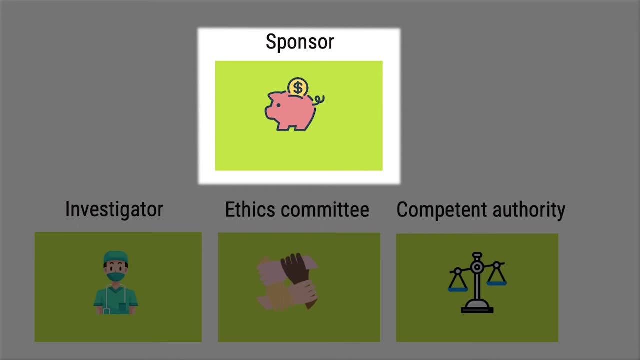 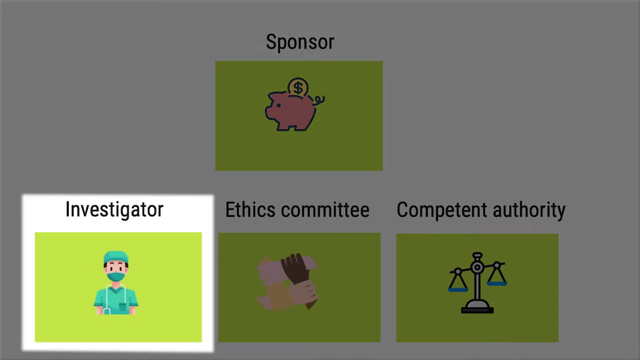 and their ethical responsibilities. To summarize, the sponsor is ultimately responsible for the clinical investigation, the quality planning conduct, as well as ensuring appropriate communication with the regulatory authorities, such as the competent authority. The investigator is responsible for the day-to-day conduct of the clinical investigation and the investigator 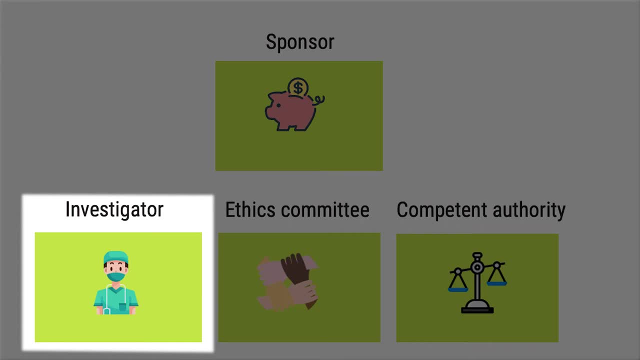 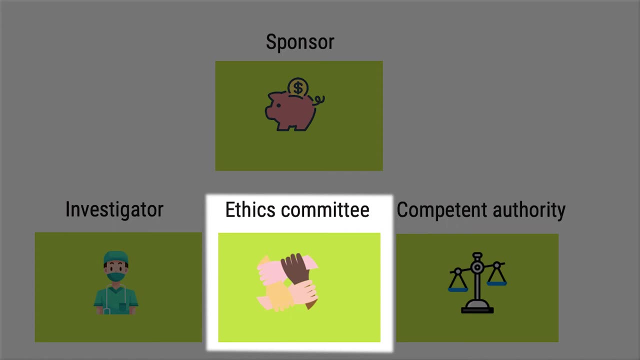 must be qualified by education, training and experience. The ethics committee is the independent body that is responsible for the clinical investigation and the investigator should give opinions on the ethical and scientific matters of the clinical investigation, And the competent authority is the regulatory body that acts on behalf of the government to ensure. 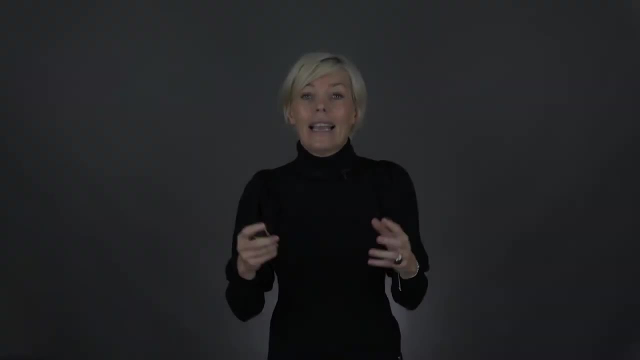 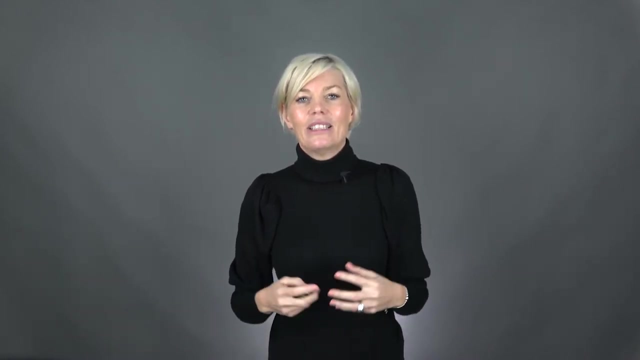 that the legal requirements are applied. Any of the stakeholders can, unfortunately, and often without knowing it, breach the requirements outlined in the GCP and ISO 14155 standard. Much of our work as clinical research professionals is to know that the GCP and the 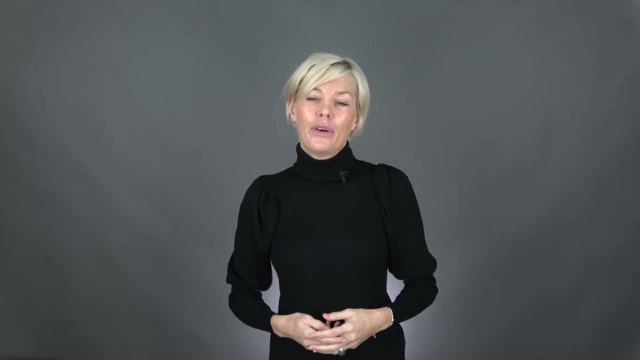 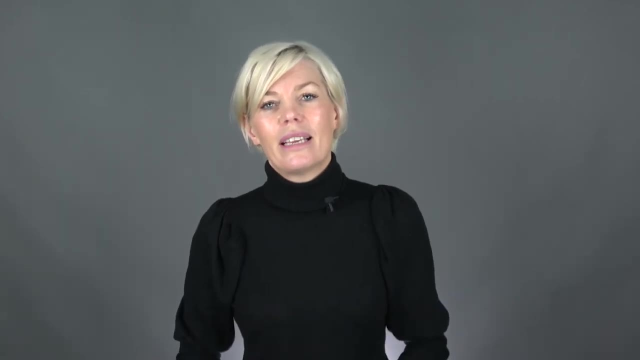 ISO standard are so well-organized that we can anticipate and avoid making these mistakes. In the full course, we talk more about the breach of GCP, serious protocol deviations and how to make sure that you can avoid this. Now that you understand the importance of the 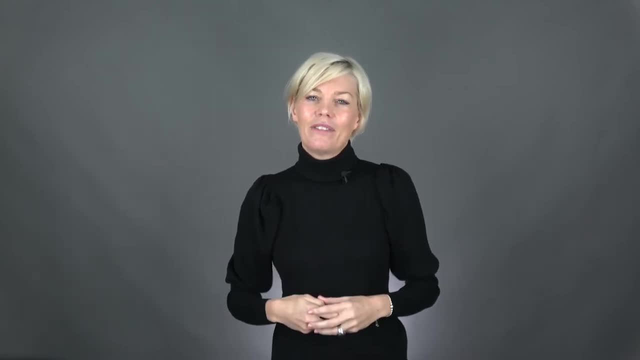 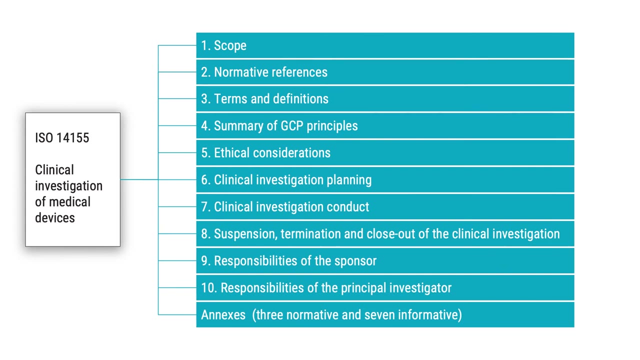 ISO 14155,. let's look at some of the specific sections and its requirements. The standard released in 2020 has 10 clauses and 10 annexes: three normative annexes and seven informative. It's almost twice as long as the previous standard version. It starts by providing: 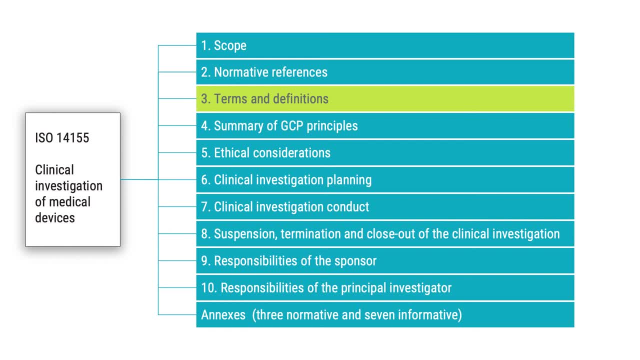 an overview of terms and definitions, and there are quite a few of them- actually 55.. I can really recommend to carefully read them, since it's very useful that you use the correct term that is widely accepted and well-defined. What is new in the 2020 version is a summary of the GCP. 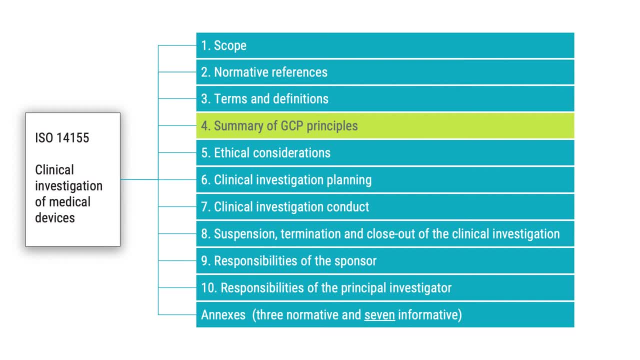 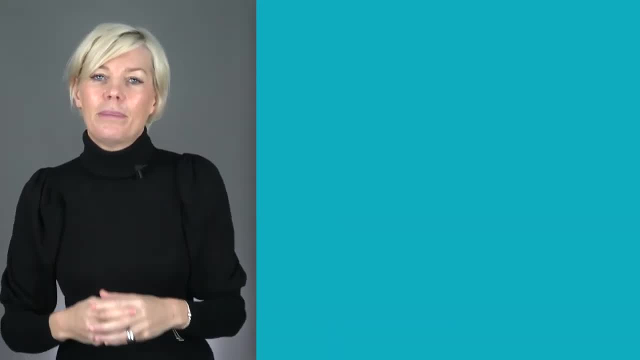 principles which have been aligned with the ICA's GCP principles, And this is presented in clause four. This is an excellent summary. The 13 GCP principles are summarized and start with that. a clinical investigation must be conducted in accordance with the ethical 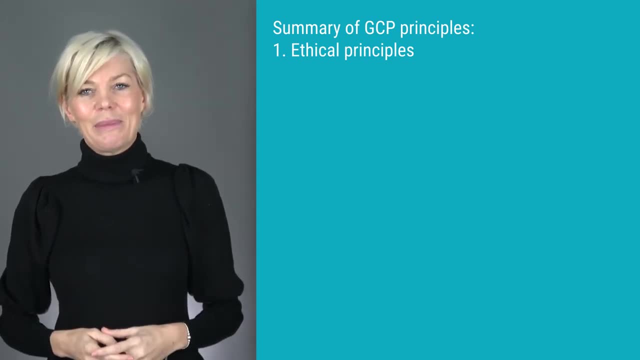 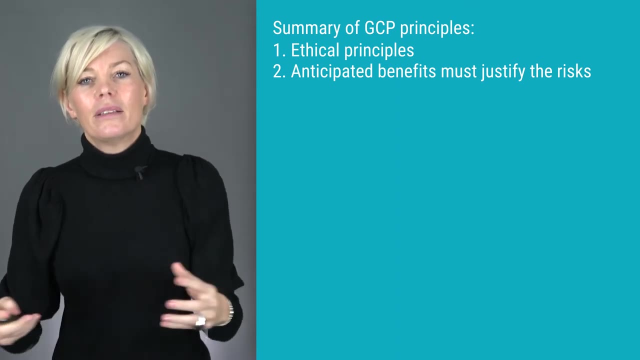 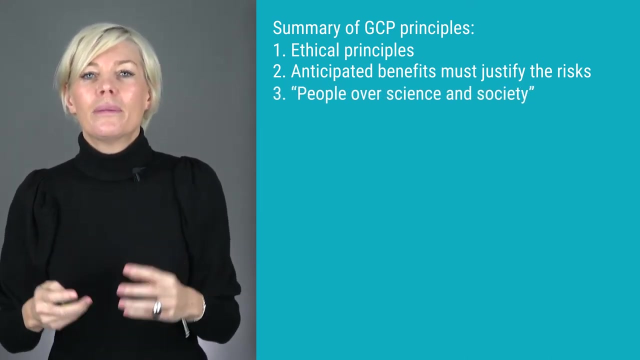 principles that have their origin in the Declaration of Helsinki. You also have to ensure that the foreseeable risks are weighed against anticipated benefits for the individual subject as well as the society. The rights, safety and well-being of human subjects are the most important considerations. 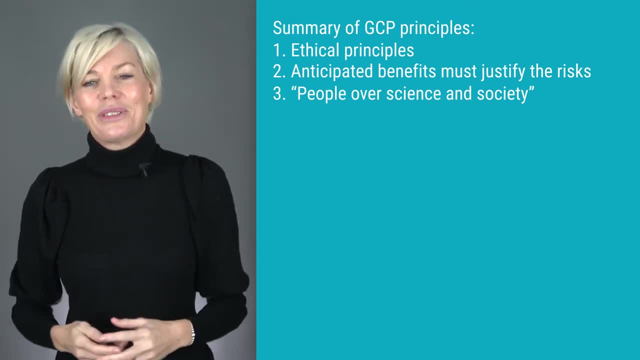 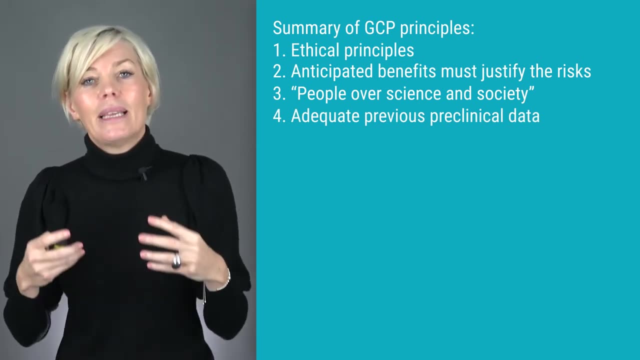 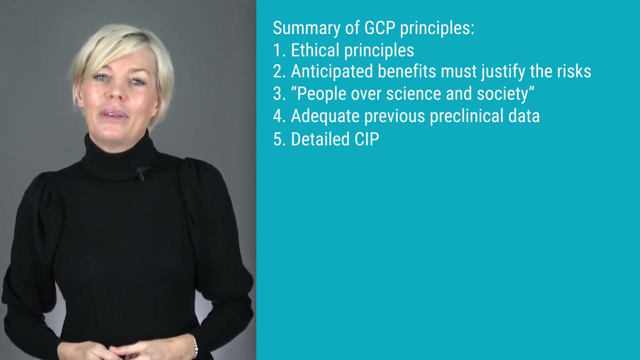 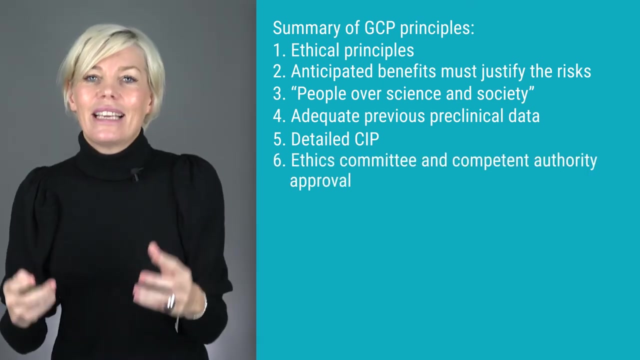 And should prevail over interests of science and of society. The available preclinical and clinical information on the investigational device should be adequate to support the proposed clinical investigation, And the clinical investigations must be scientifically sound and be described in a clearly detailed clinical investigation plan, the CIP, The clinical investigation. 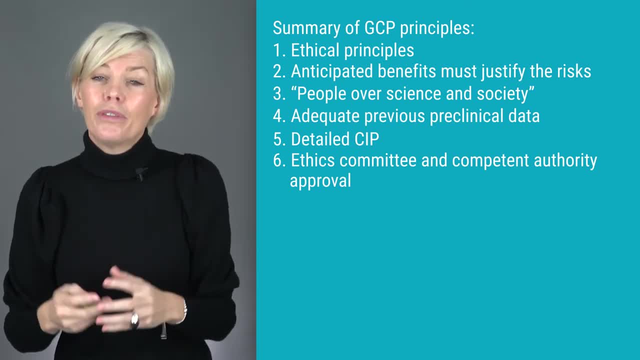 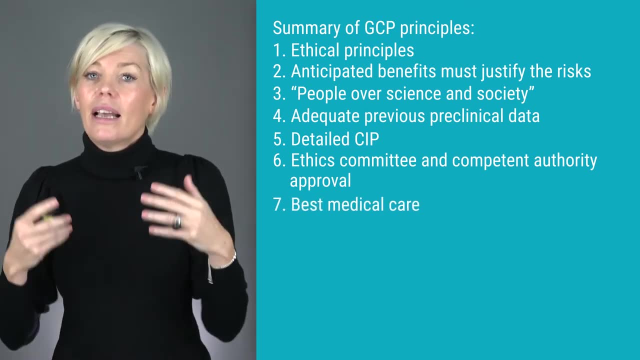 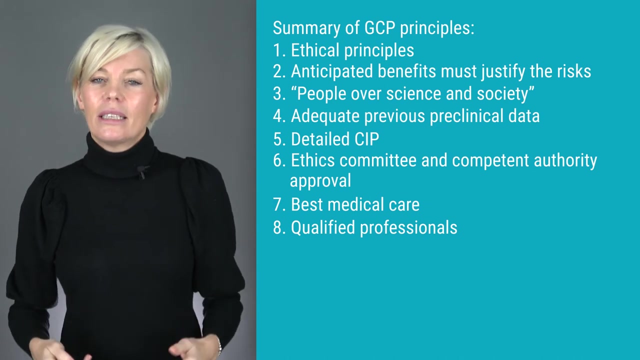 must receive prior ethics committee approval and approval from the regulatory authorities where needed. The medical care given to the subjects and the medical decisions made is the responsibility of a qualified healthcare professional. Each person involved in designing, conducting, recording and reporting a clinical investigation must also be qualified by education. 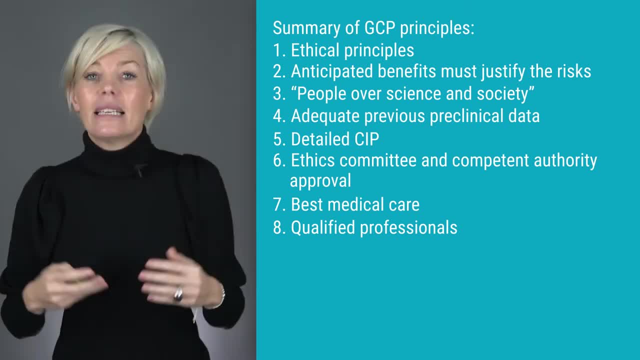 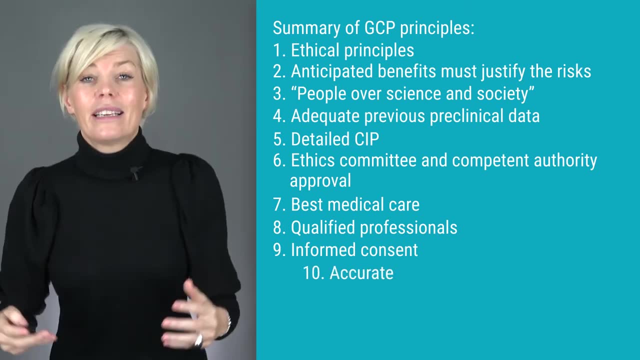 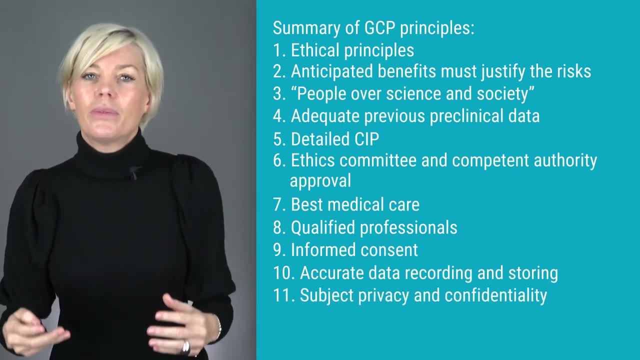 training and experience to perform their task. Each subject should freely give an informed consent prior to the participation in the clinical investigation. All clinical investigation-related information should be recorded, handled and securely stored. The confidentiality of records that could identify subjects must be protected and respect the privacy and confidentiality. 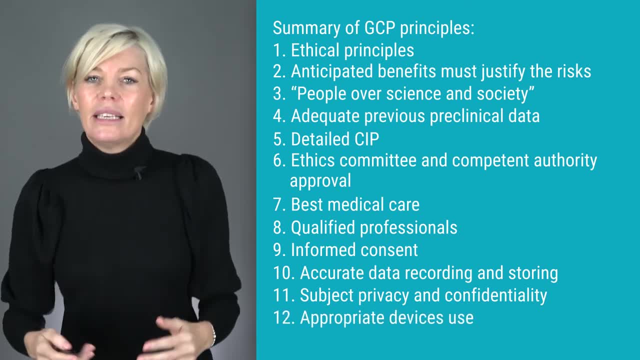 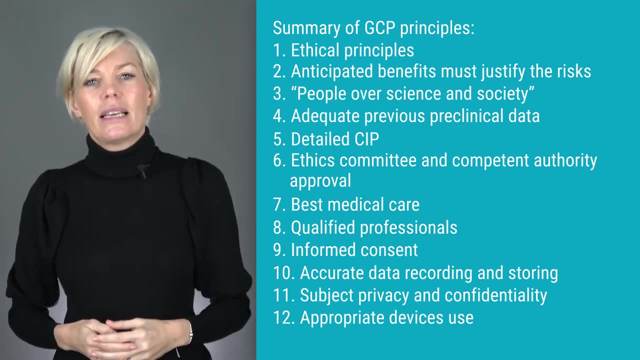 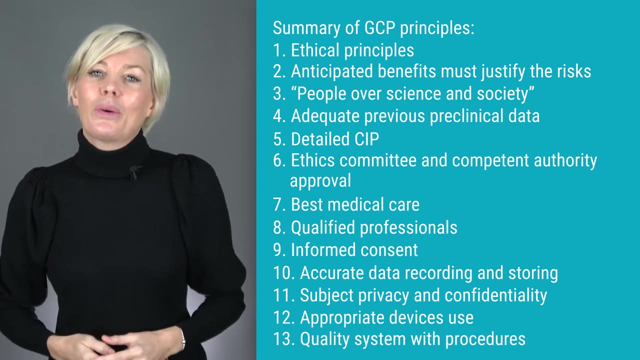 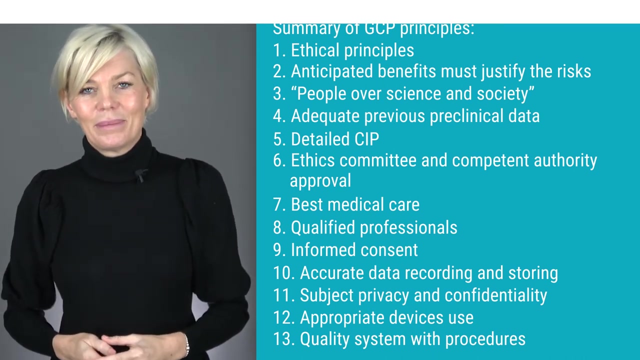 rules. Investigational devices must be designed, manufactured, handled and stored correctly, and they must be used in accordance with the approved clinical investigation plan and the IAB and manufacturer's instructions for use. And finally, there should be a quality system in place with procedures that ensures the quality of every aspect of the clinical investigation. 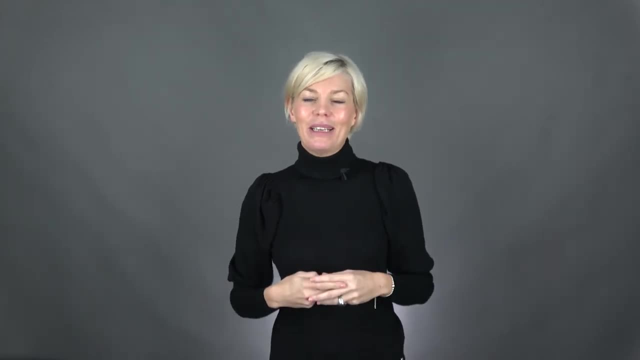 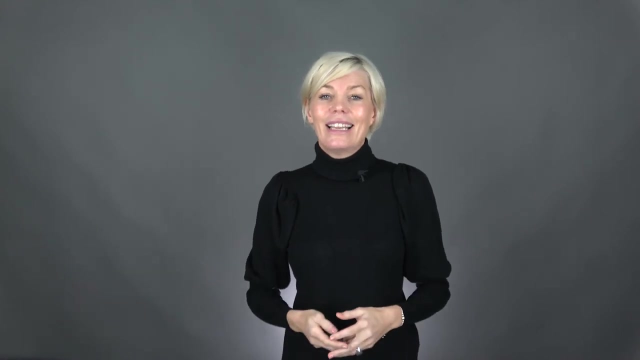 I also want to show you that, while clinical investigations of medical devices have many similarities to clinical trials for pharmaceuticals, the regulatory evaluation of devices is distinct to that of drugs And there are critical differences in the way that device studies are designed and executed. Let's look at this. So clinical research is broken up into a series of phases. 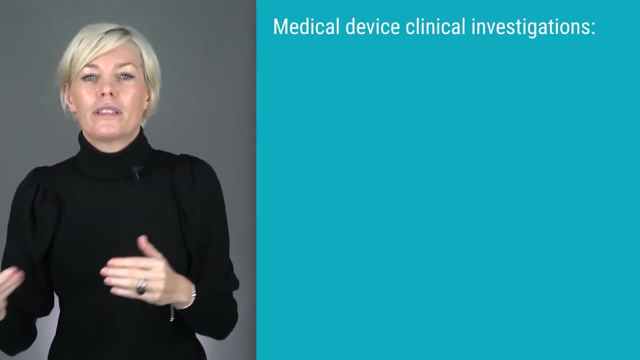 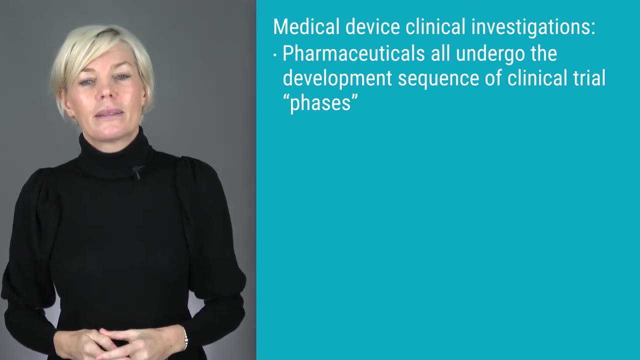 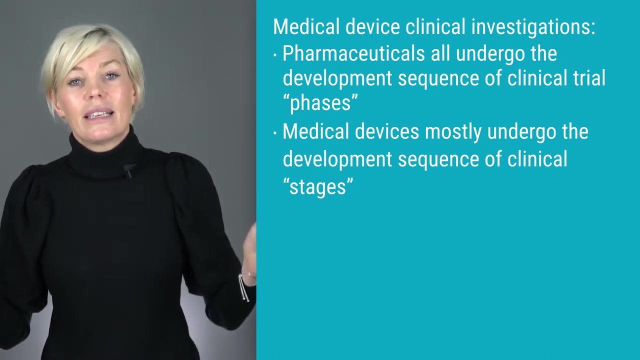 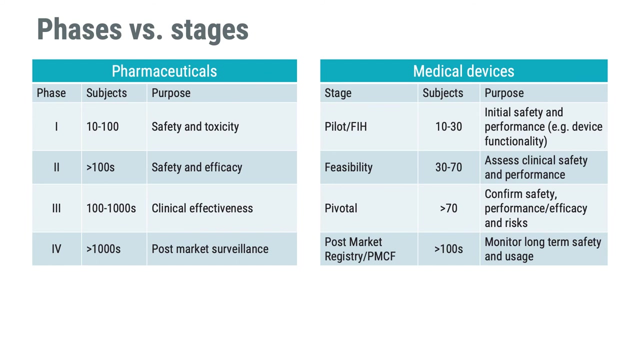 Each with a distinct purpose. phase I to phase IV Pharmaceuticals must undergo the full clinical trial phase sequence before market release. For medical devices, the sequence is similar. However, most medical devices will go through clinical investigation stages instead of phases. This table provides a side-to-side comparison of pharmaceutical trial phases versus medical 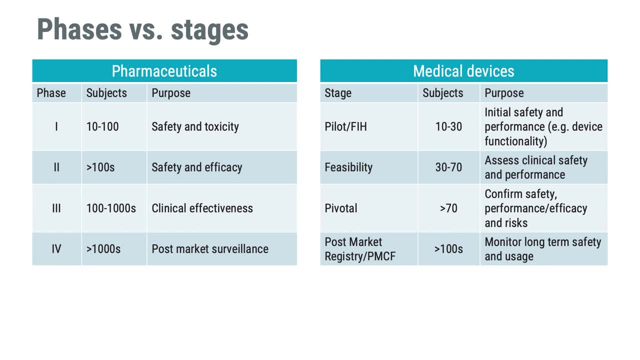 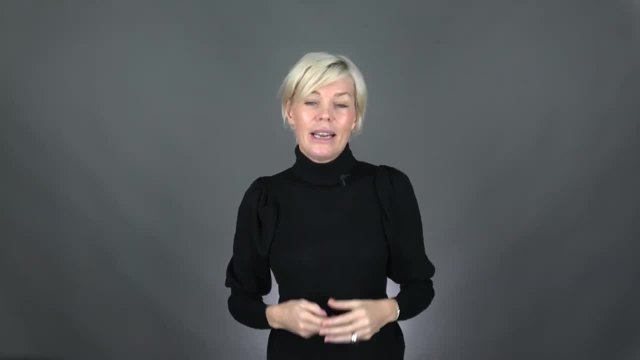 device stages. It also shows the main differences between the two. The first is the clinical, between the different phases and stages for drugs versus devices. I know it contains a lot of information and in the full course we review this stage by stage. And finally, I would like to end this short course by speaking a bit. 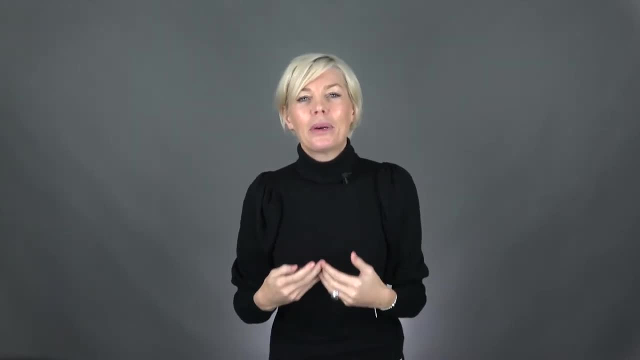 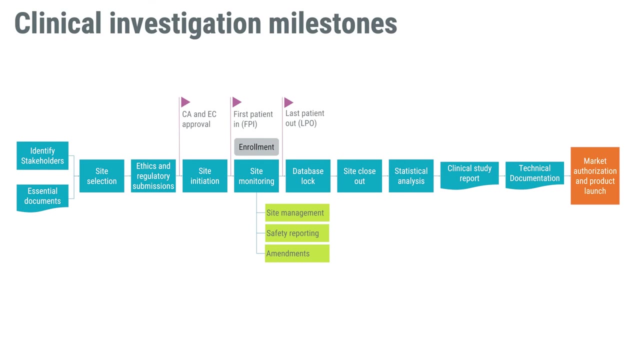 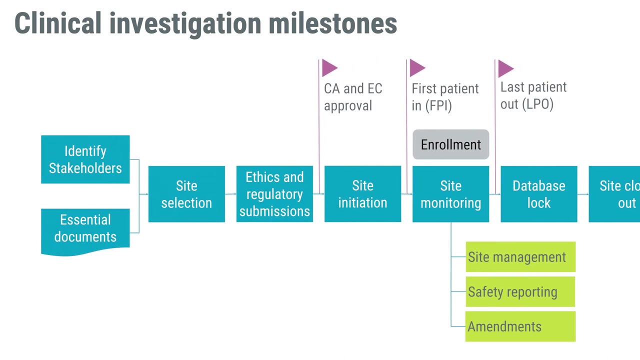 about the clinical development process and the importance of carefully preparing a clinical research budget and to monitor costs and timelines. I have prepared this flow chart outlining critical steps that you need to adequately plan and execute towards. This is, of course, simplified and there could be many more pitfalls. 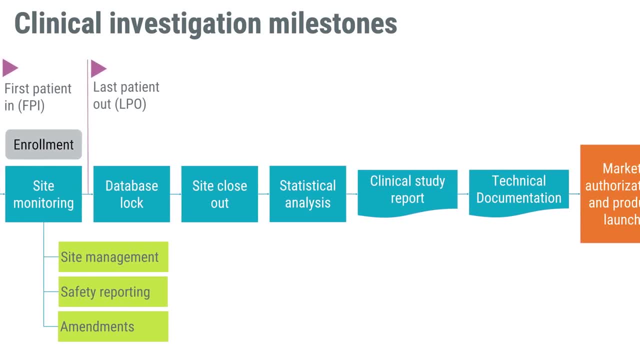 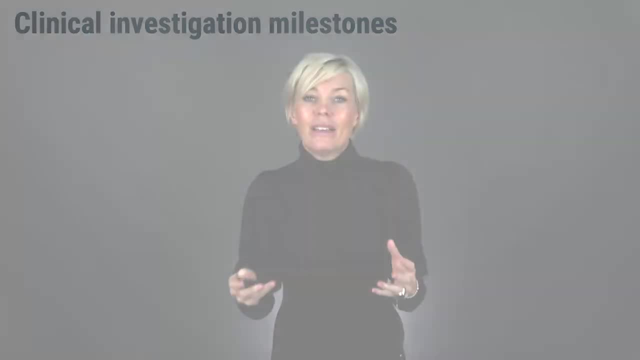 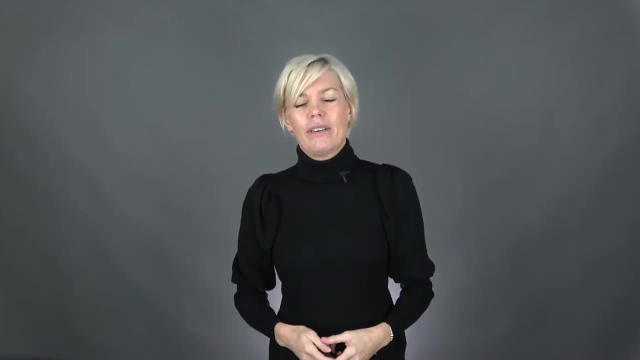 during this journey, We will review all of these steps in the full course and you will learn how to anticipate some of these challenges and avoid some of the pitfalls. Clinical investigations are notorious for their complexity. They typically take many years to reach completion and are often very costly. 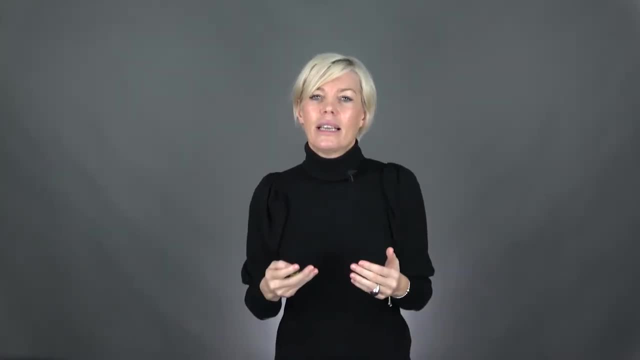 But in this course you will see that there are several actions that you can take to optimize the process And make sure that you set up a successful study and even save money. We have now come to the last part And with all that you have learned, you have probably realized that you 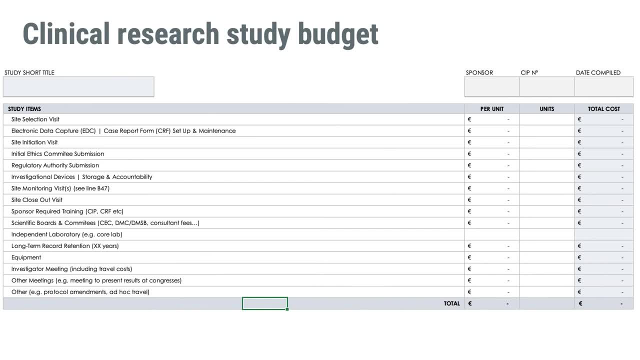 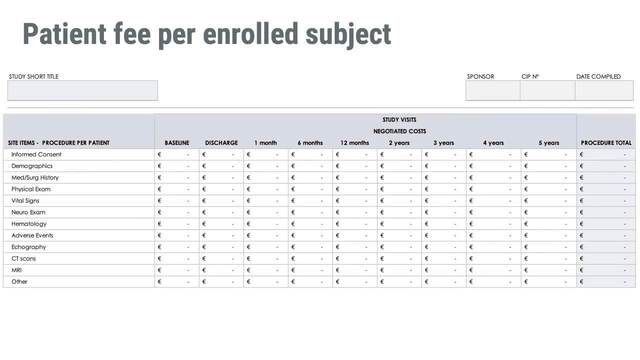 need to build a solid clinical budget to convince your manager, the sponsor and possibly investors about the project's feasibility. You will need to identify the key cost parameters for your clinical research project. It is also important to make sure that you keep an eye on the differences.